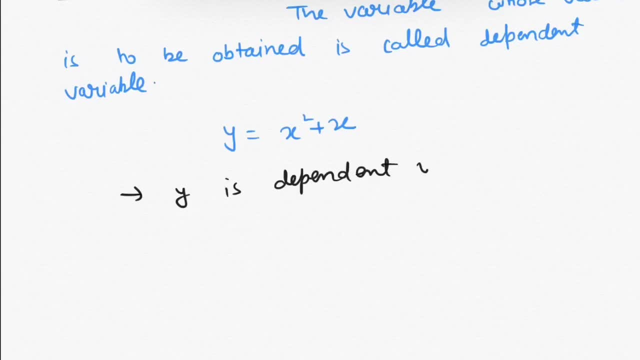 And x is independent variable. Now let us see another example. z equals to x square plus y square Here. in this equation, z depends on the values of x and y. So z is dependent variable And x and y are independent variable. 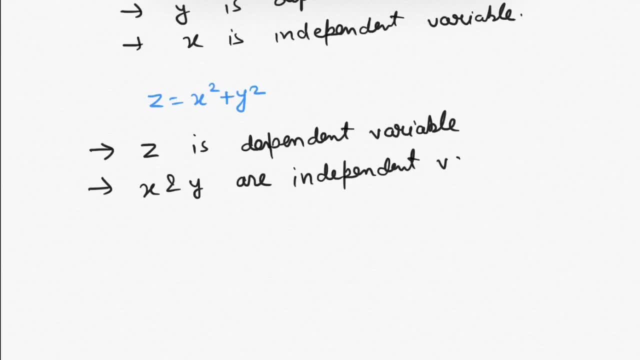 And x and y are independent variable. And x and y are independent variable. I hope everything is clear to you till now. Now let's proceed to the main topic of today's video. You all heard about two types of differential equation: Ordinary differential equation and partial differential equation. 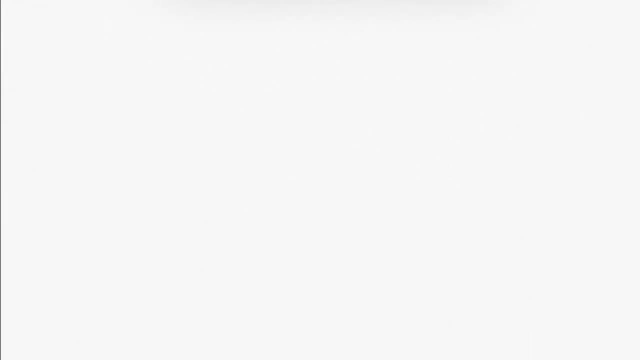 So there are two types of differential equation. One is ordinary differential equation- ODE- And another is partial differential equation- PDE. In ODE there is only one independent variable, One independent variable, While in PDE there are more than one independent variable. 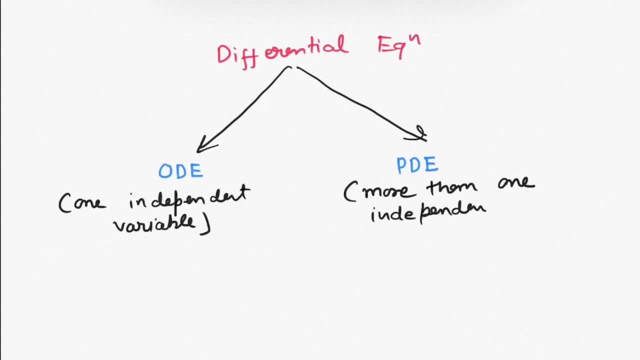 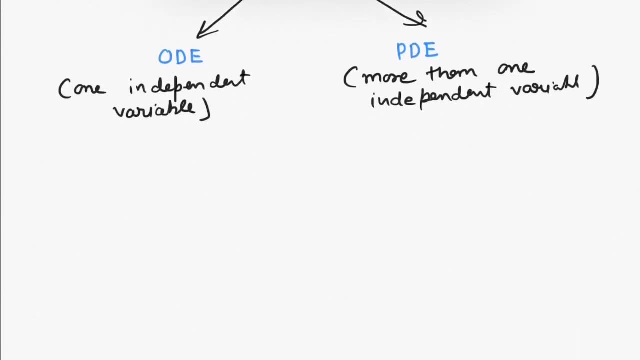 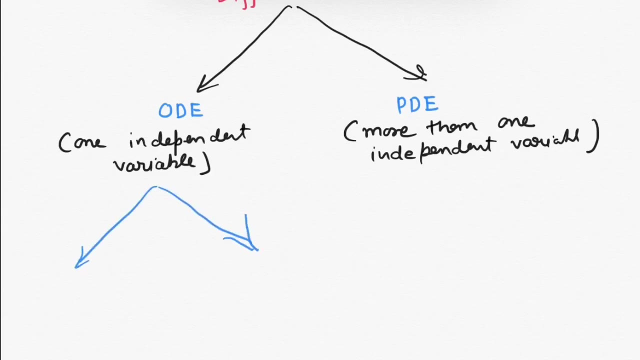 While in PDE there are more than one independent variable, In ODE there is also two categories. In ODE there is also two categories: When there is one dependent variable, When there is one dependent variable, When there is one dependent variable. 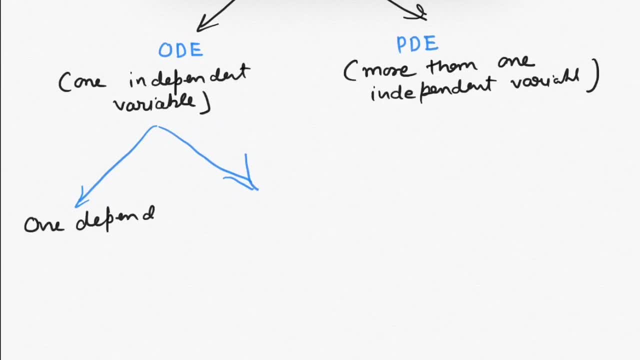 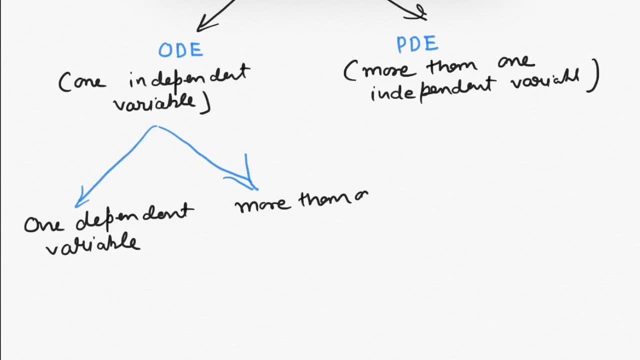 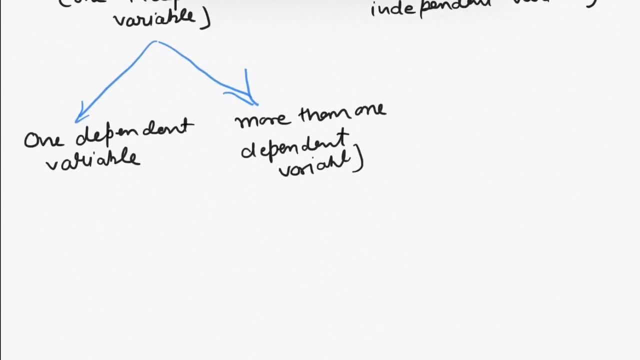 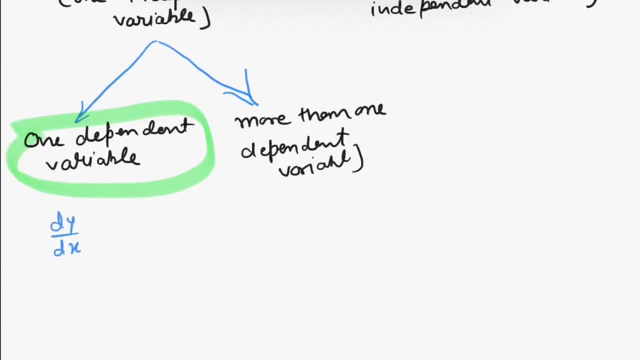 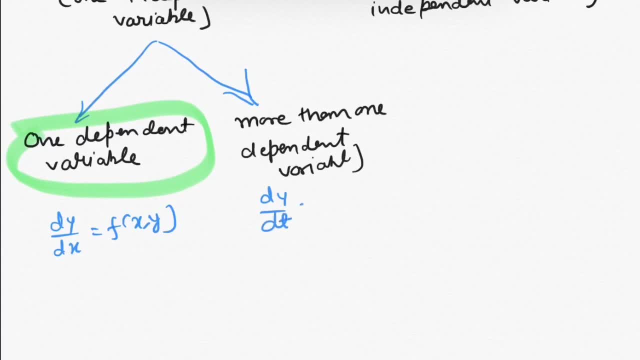 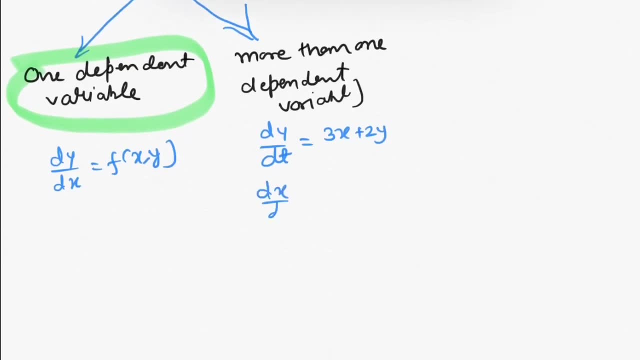 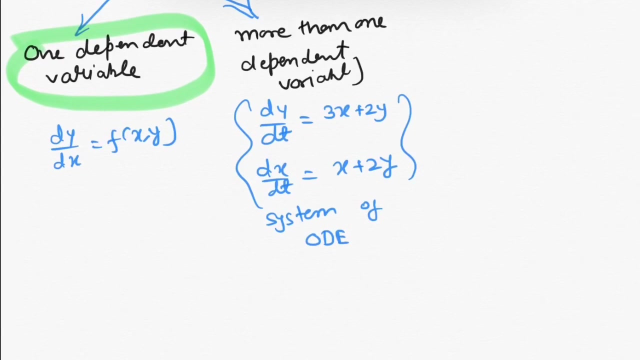 When there is more than one dependent variable. When there is more than one dependent variable to 3x plus 2y, and dx over dt equals to x plus 2y. okay, this is system of system of ode. okay, and here x and y both are function of t. okay, now let us see how pd is. 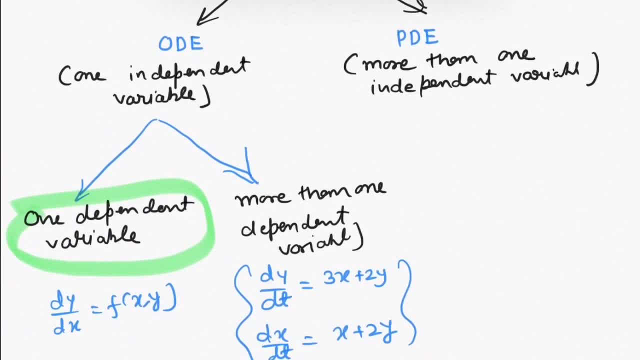 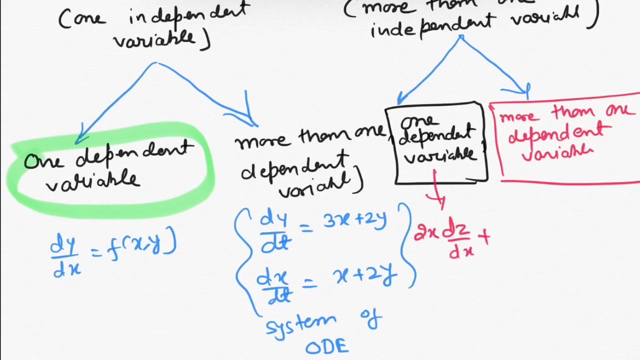 categorized okay. pd is also categorized in the same manner when: when there's only one dependent variable, one dependent variable and when more than one dependent variable: okay. one of its example is 2x. dz over dx plus phi y dz over dy equals to 1- okay, and here z is a function of 2z. close. 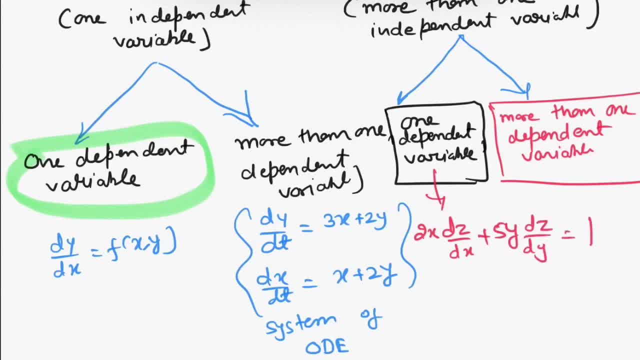 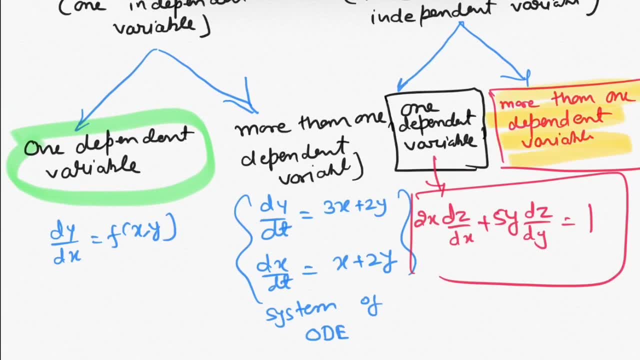 out now. let'sณy nyDn vn and LAUGHTER zформatn of x and y. in this category, You will get a system of partial differential equation. Okay, you will see its example more often in your PhD research work. Okay, Now this. 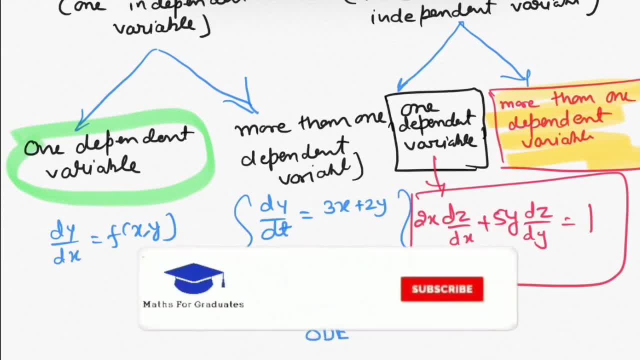 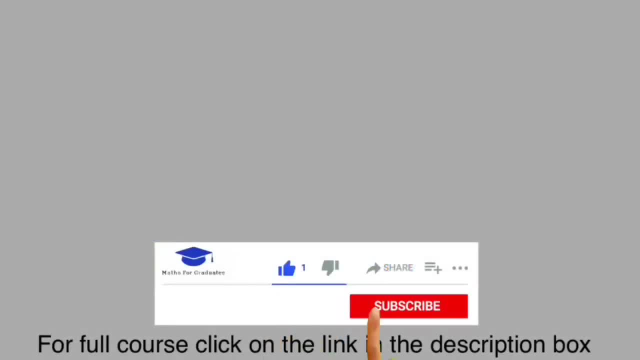 video ends here. If you find this video informative, then show your support by subscribing the channel, Thank you. Thanks for watching you.